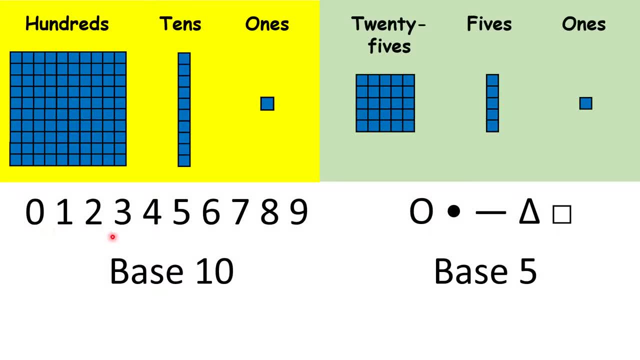 So we use 10 digits to represent numbers, so we can say that our number system is base 10.. That means that when you have 10 of something, you move to the next place value column along. or, putting it a different way, that each place value is 10 times larger than the place value. 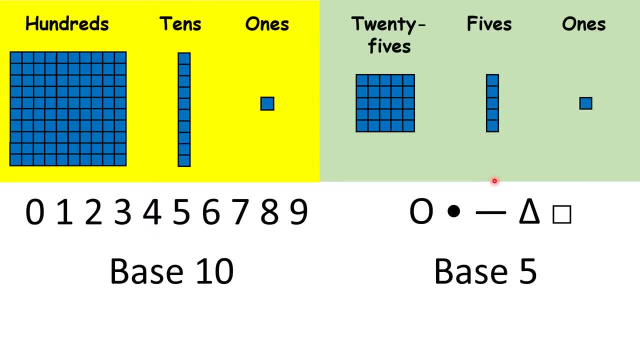 before it. With the Rigglesfordian number system I have 5 symbols, which means that I have a base 5 number system. That means that when I have 5 of something I move to the next place value column along, so each place value is 5 times larger than the place. 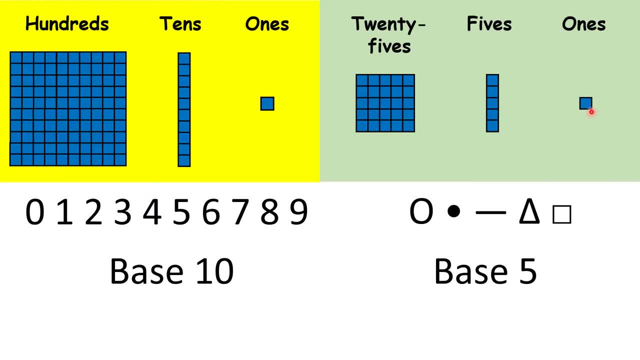 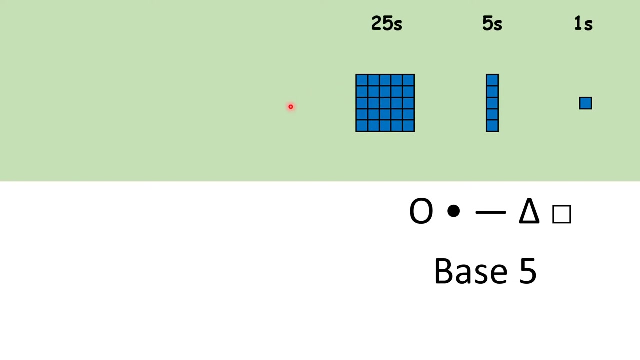 value before it. So rather than units, tens and hundreds, I have units 5s and 100s. Now we know that after hundreds we have thousands, ten thousands and so on. But what is the next place value after 25s in the Rigglesfordian number system? Well, because my number system 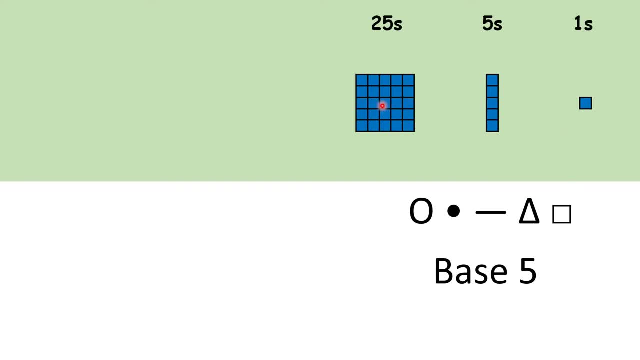 uses 5 symbols. each place value is 5 times larger than the one before it, so we can work out 25 times 5.. That gives us 125, so our fourth place value column is the 125s. So how can we work out what we have next? We need to work out 125 times 5.. So that means 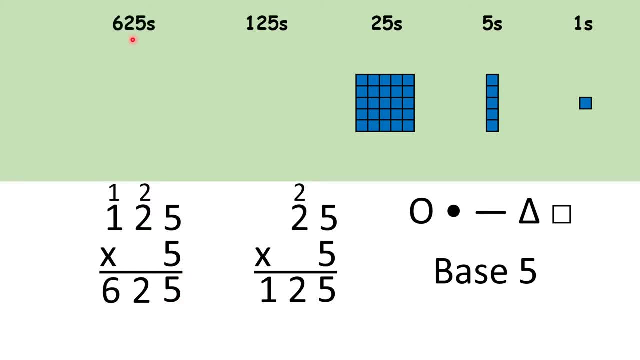 our next place value represents multiples of 625.. 625.. 625.. 625.. 625.. 625.. So how is Rigglesfordian place value similar to and different from normal place value? Well, the place values represent different quantities. but just as with our place value system, we can keep going along the place values by multiplying by 10,. in the Rigglesfordian number system, we can go along the place values by multiplying by 5.. 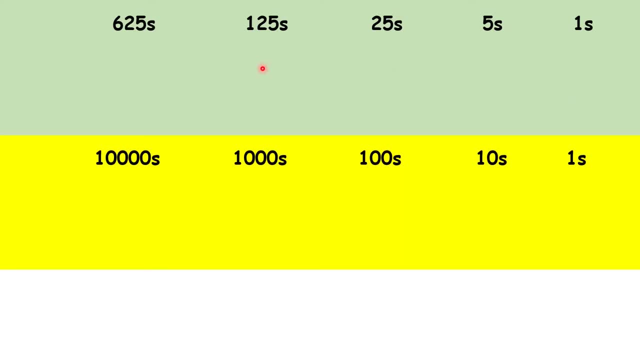 So here we have our Rigglesfordian place value at the top and our normal place value at the bottom, So we have units 5s and then we have 25s, because 5 times 5 is 25.. 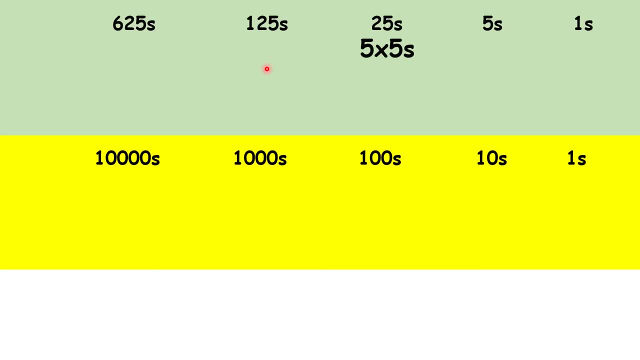 Then we have 125s, because 5 times 5 times 5 is 125.. Then we have 625.. Then we have 5s, because 5 times 5 times 5 times 5 is 625.. So that's place values with base 5.. 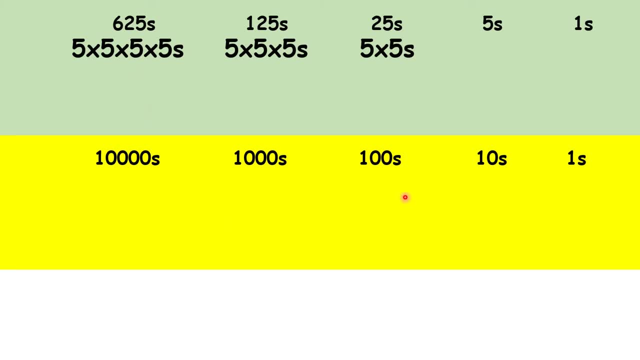 But though what the place values represent is different, it's a similar idea to what we do with our normal base 10 system. We have units, then 10s, then 100s, because 10 times 10 is 100.. 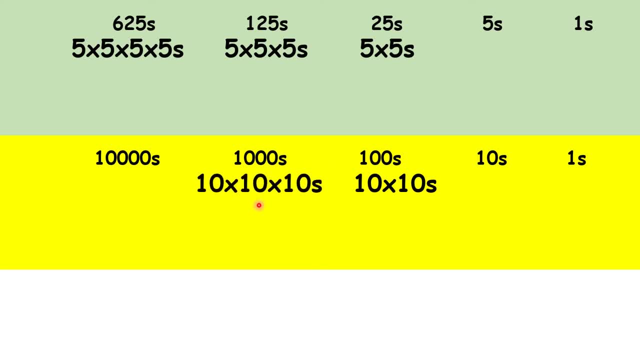 Then 1000s, because 10s is 100. Then 10s, because 10 times 10 times 10 times 10 is 1000. Then 10 thousands, because 10 times 10 times 10 times 10 is 10,000.. 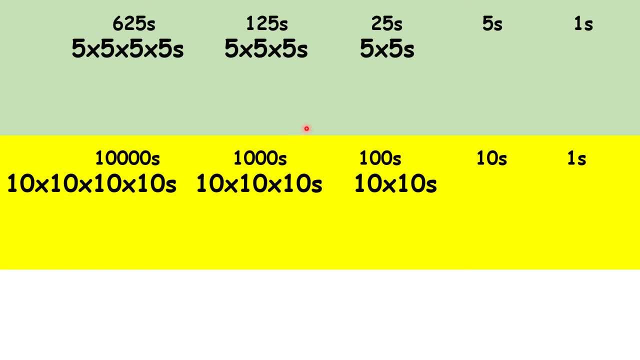 So we can start to think about place values in a different way. Rather than thinking of numbers, let's think of powers. So for 25, or 5 times 5,, we can say 5 squared that's 5 times itself. 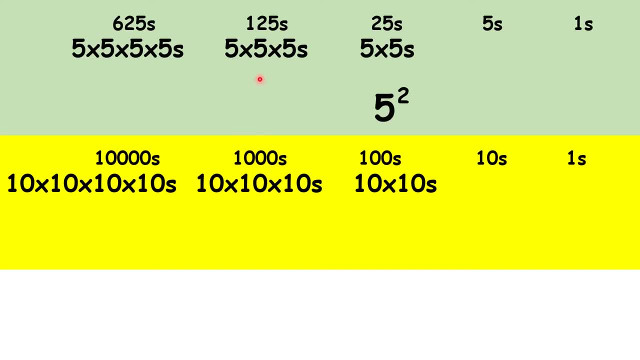 Then for 125, or 5 times 5 times 5,, we can say 5 cubed, And for 625, or 5 times 5 times 5 times 5, we can say 5 to the power of 4.. 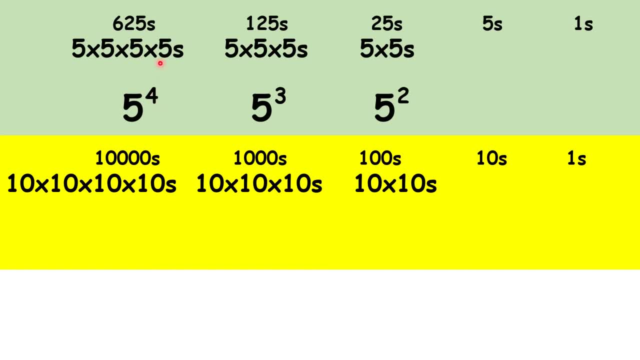 You might not have seen to the power of 4 before, but you can probably work out what it means. Well, notice that we can. We can do the same with base 10.. Rather than writing 100s as our place value heading, we could write 10 squareds. 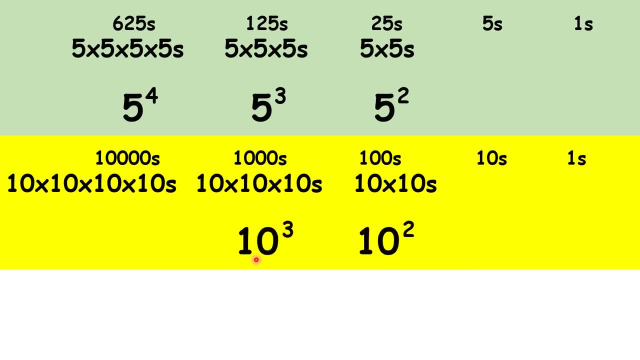 Then, instead of 1000s, we could have 10 cubeds. Then, instead of 10 thousands, we could have 10 to the power of 4s. One other thing you'll learn about powers is that any number to the power of 1 is just itself. 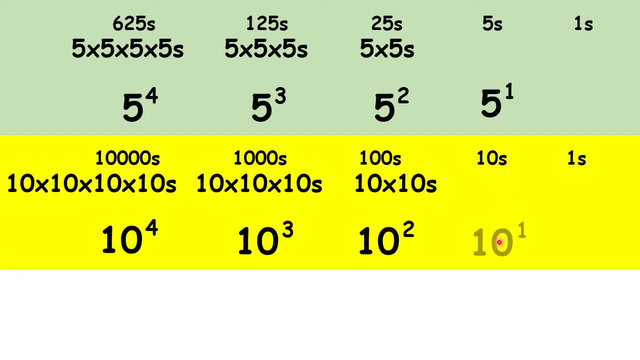 So we can have 5 to the power of 1, and 10 to the power of 1, for our second place value columns. Another thing you'll learn is that any number to the power of 0 is 1.. So we can have 5 to the power of 0, and 10 to the power of 0, instead of our units.